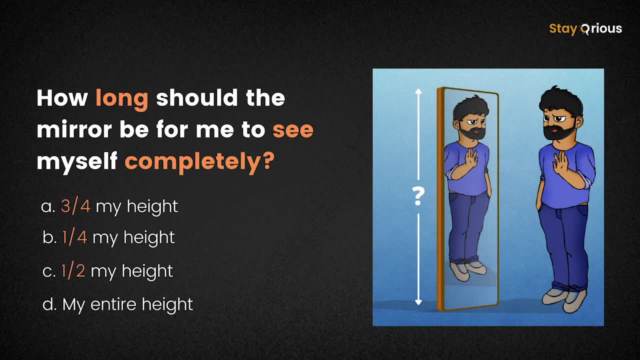 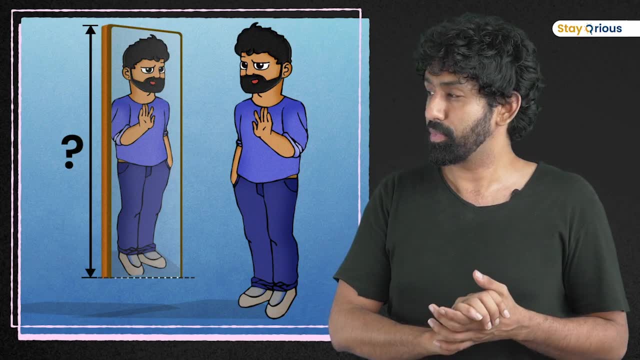 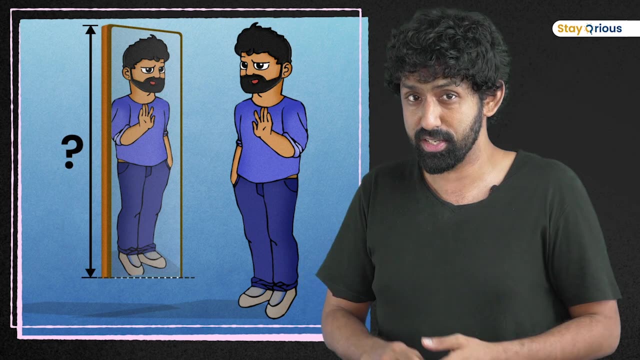 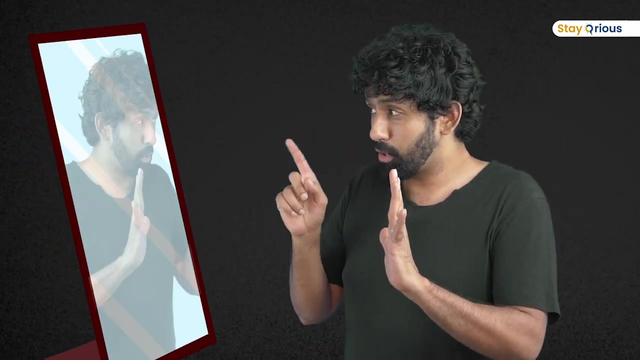 Now to answer that question. we'll have to understand how images form in a mirror. How exactly is it forming? And then we can get to the bottom of this. So let's jump in. Let me ask you a question. If I take my hand like this and keep it right, I can see my hand directly. But I can 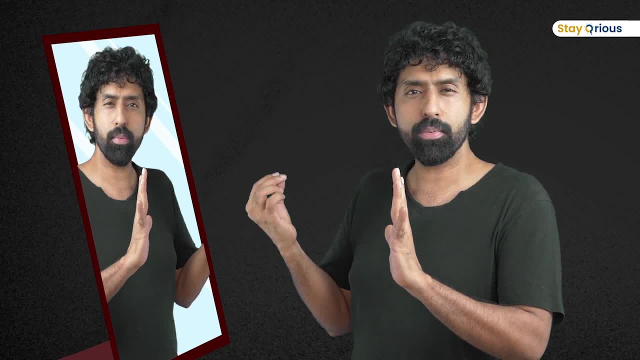 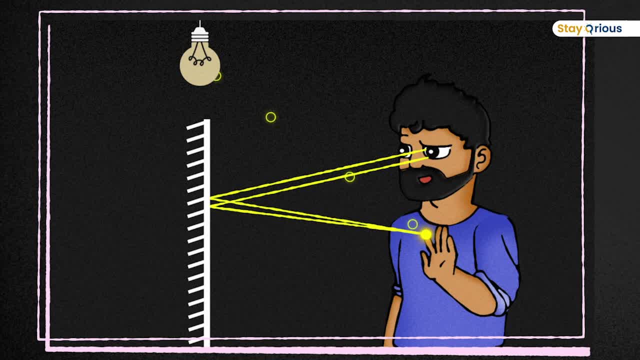 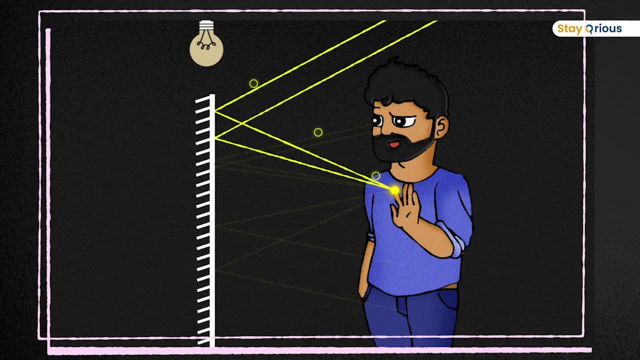 bouncing off my hand, bouncing off the mirror and then hitting my eye right. Many of them are bouncing off the hand, going somewhere else. They don't help me see. Many are bouncing off the mirror but will never reach my eye. Why is that? Because of all the photons that bounce off the 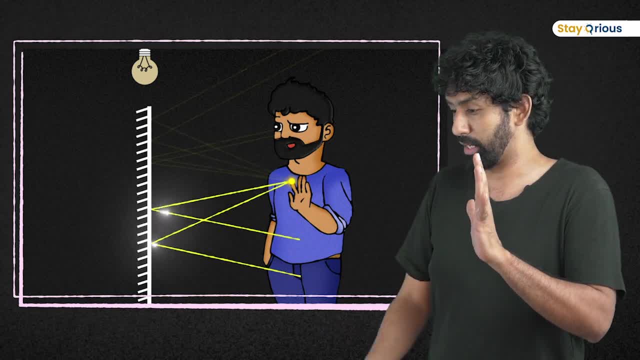 mirror. not all of them will end up in my eye, right? Some of them are bouncing down, going that way. Some are bouncing here going that way. Yeah, all of them. don't hit my eye unless it hits my eye, And then I can see myself fully in that mirror. So I can see myself fully in that mirror. 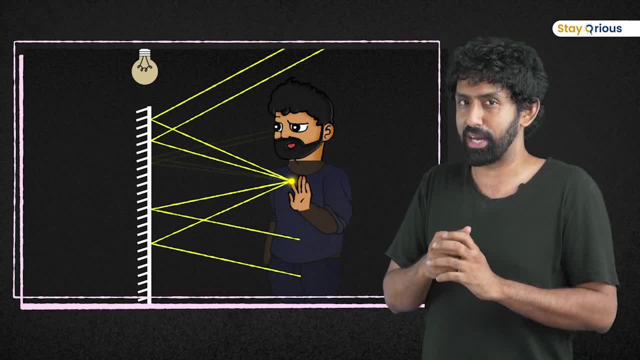 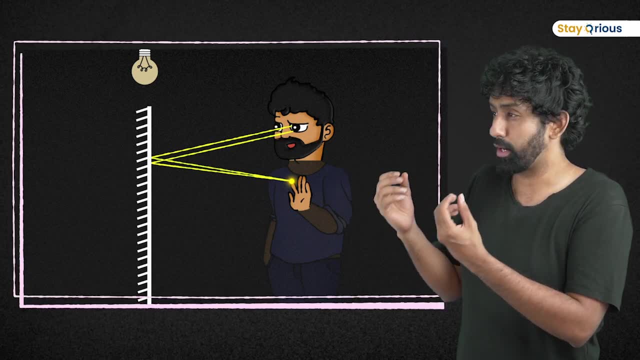 It doesn't help me see a point on my hand. Let's take one point on my hand, right? So only those photons right that hit the mirror and bounce beautifully. right, All of them are bouncing. according to the law of reflection, Angle of incidence equals angle of reflection. all of them. 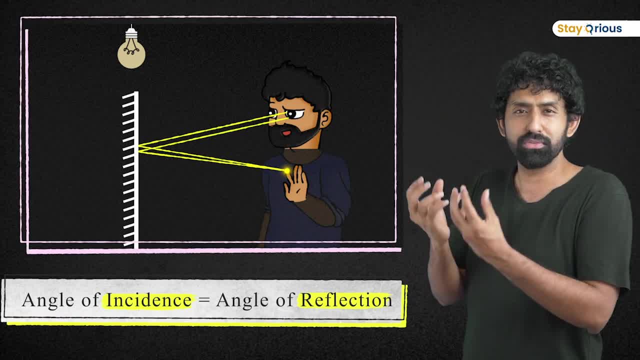 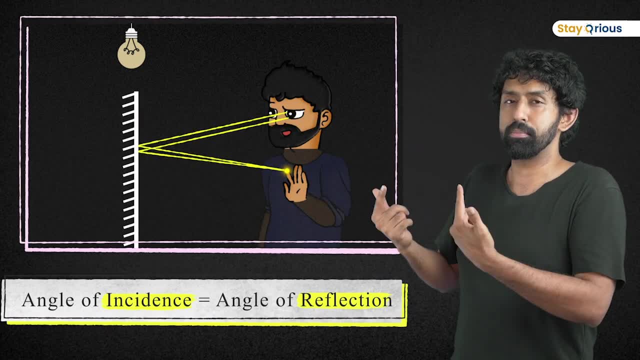 And some small person, if some 1 billion left, some I don't know very small percentage- are hitting the mirror in such a place such that it bounces and comes into my eye right. Those are the ones that tell me: oh, there's an image of this point, And where do we go from here? Where do 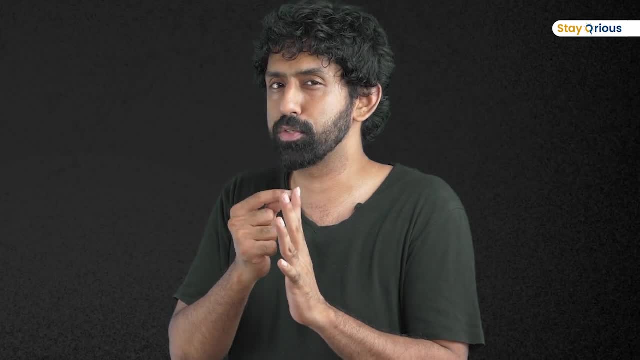 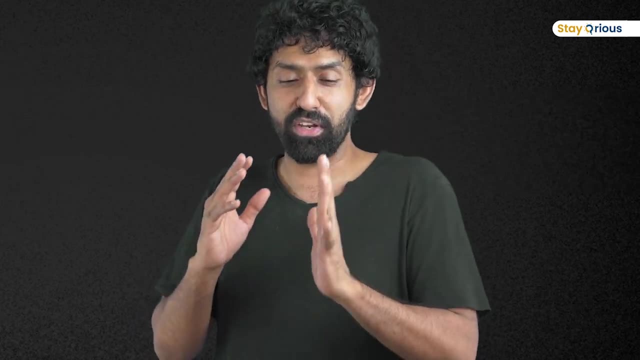 I see that image. How many rays should you consider from this point to find out where I see the image of my hand? Did you think about it? Two rays are enough. right, Because I take one ray, hit it there. I have to use. it doesn't bounce in any direction, It can't go like that or like this. 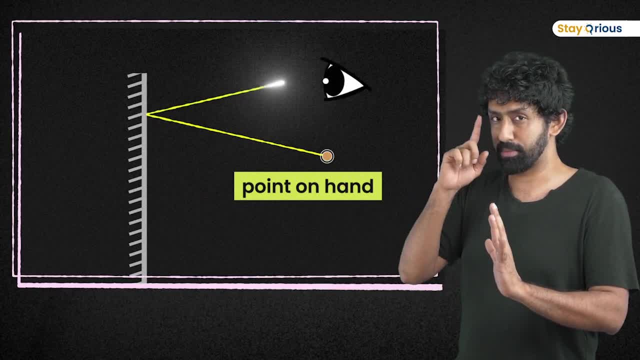 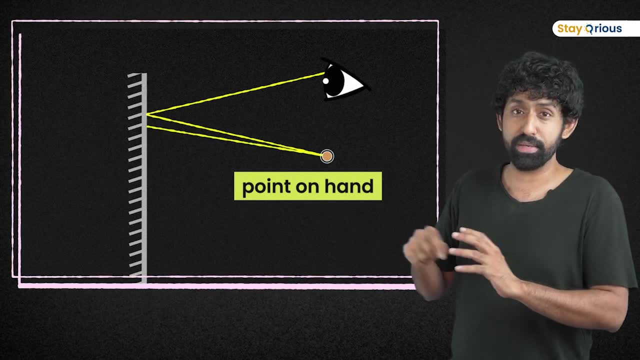 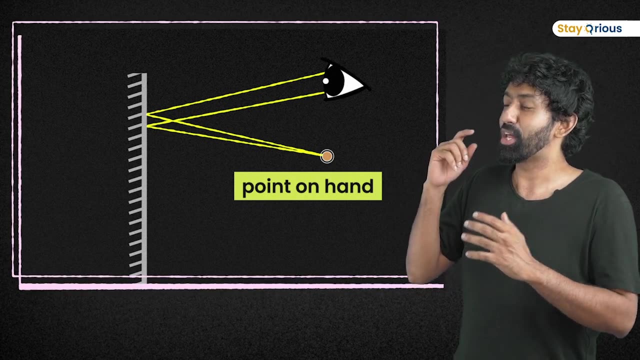 There is no spin bowling here. It has to hit and bounce right into my eye, yeah, such that the incidence equals angle of reflection. Take another ray- yeah, do the same thing again- comes and hits my eye. Incidence equals angle of reflection. Yeah, these two rays are hitting my eye. Now where will this? 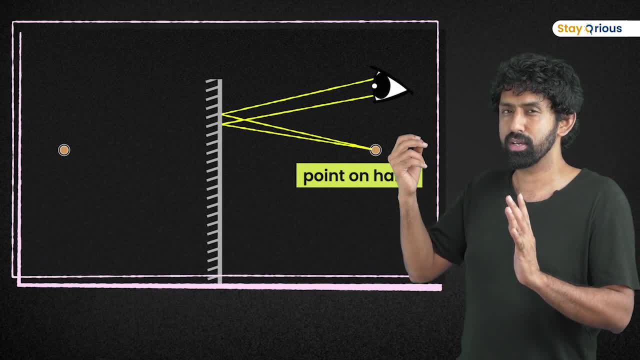 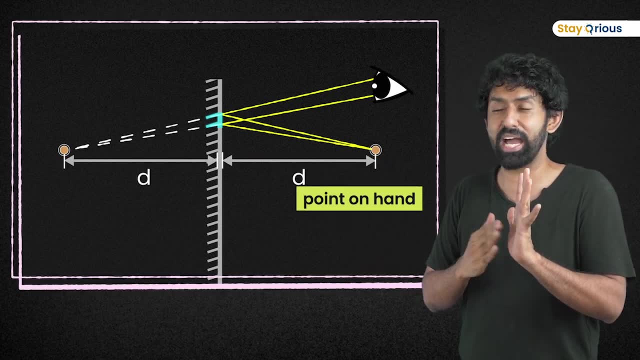 point feel like it's coming from There, right? Because my brain assumes it's coming straight from the object. So I'll see an image of this point behind the mirror, How far away behind, Exactly the same distance as my hand is from the mirror. Why is that? Go think about it. So this point. 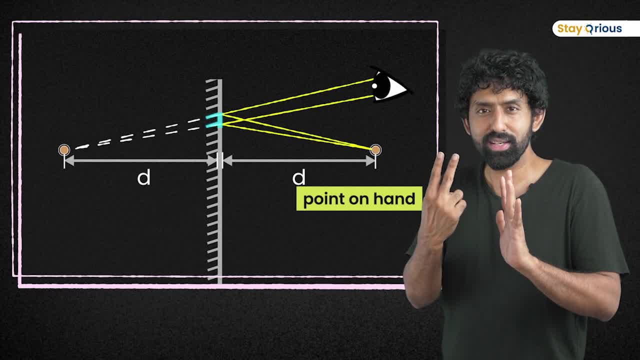 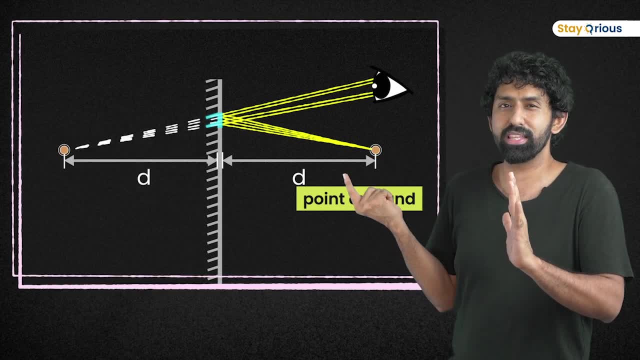 forms an image there. Now, why do I need just two rays, A third, a fourth, a fifth? whatever I draw, as you can see, will again anyway point to that point only. So if I want to know where the image of this point is, I need only two rays, right. With one, I can't do anything. 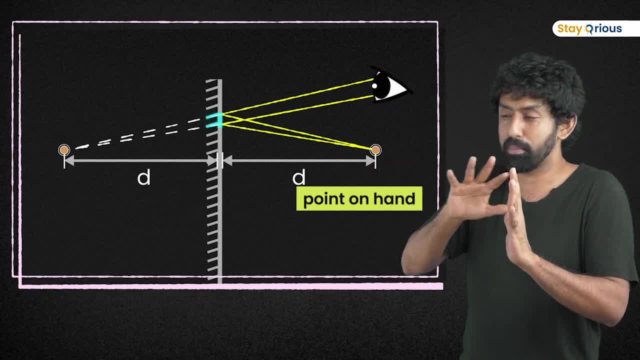 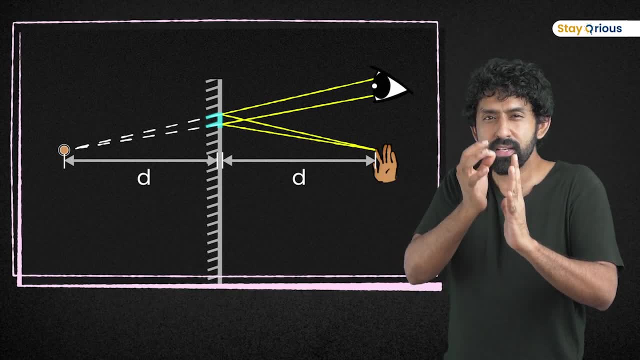 Now we know this point is there. That's how I see it: Bounces off, bounces off. the mirror hits my eye, yeah, and I see the image of this point. Now you can take every single other point, every. 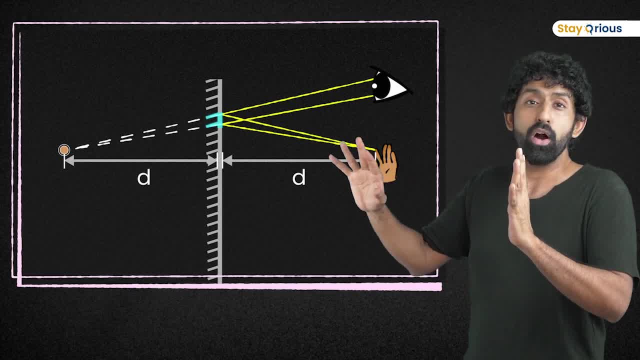 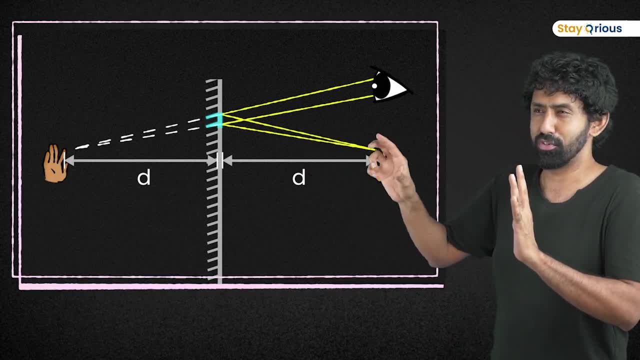 single other point. on this hand, same story happens and you see all of them bouncing off, hitting my eye from different points, and I see an image of my hand on the other side. So it's creepy right. There's a weird floating hand that I'm seeing on the other side. 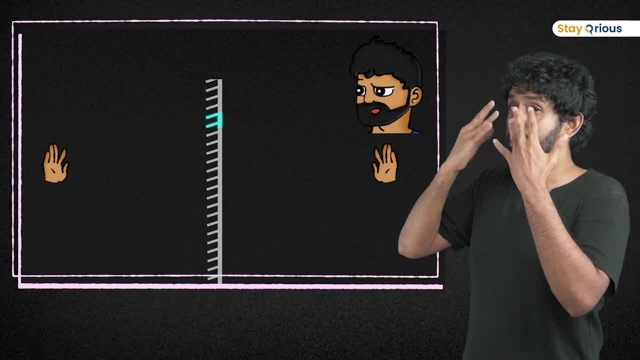 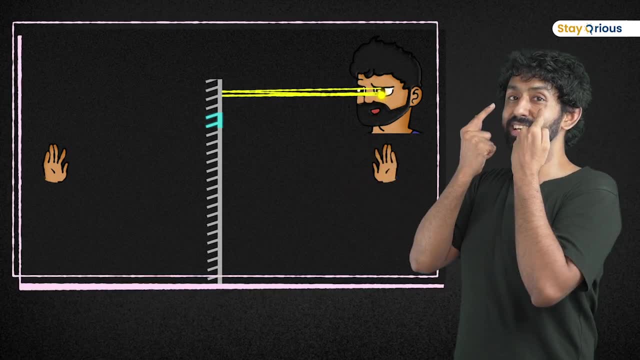 Then this: how do I see my eye Light bounces off from the light from my eye, hits my eyelid, hits my eyelashes, whatever, and then hits the mirror and then bounces back straight in. They're all hitting perpendicularly, following the law of reflection, law of- yeah, law of. 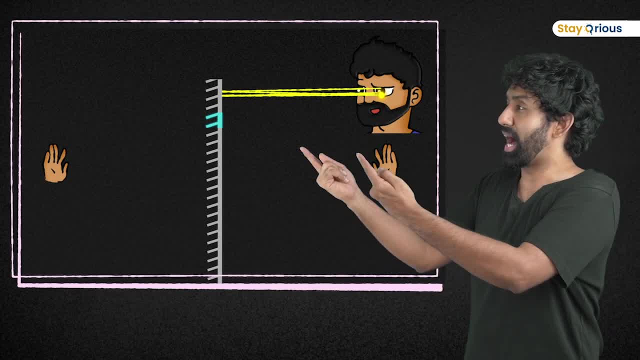 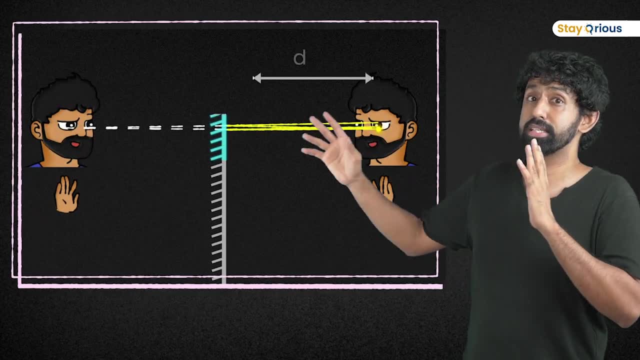 reflection. Angle of incidence is what here, That's right at zero. Angle of reflection zero comes back and hits my eye again and I see an image of my eye on the other side, exactly the same distance from where I am right. 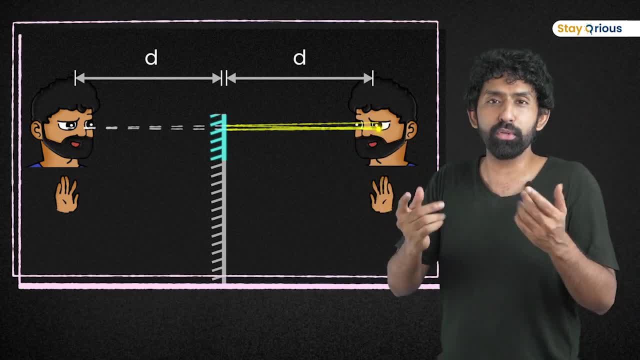 That's how far behind the mirror is. That's where it seems to be coming from. Now you can do this: My nose- same story. My neck- same story. You can keep going, and this is actually what's going on for me to 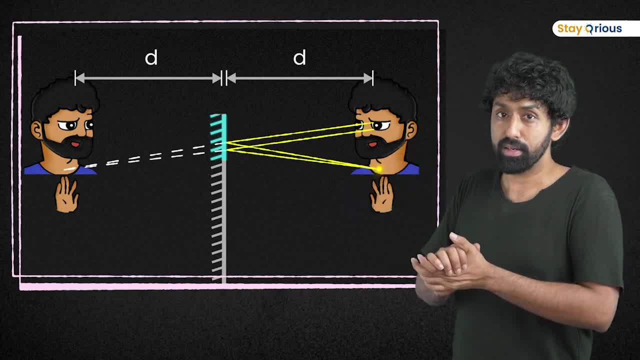 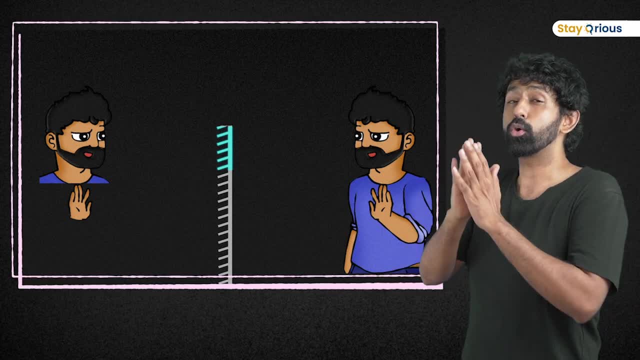 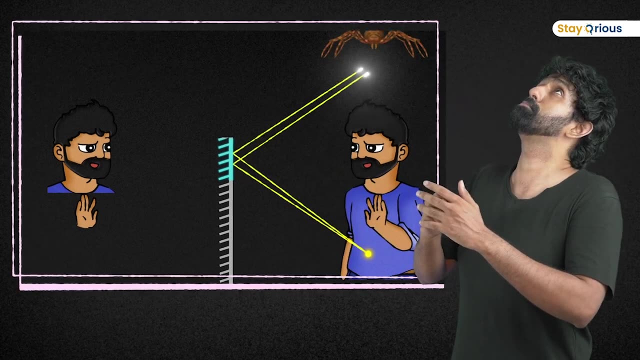 see my body in the mirror. yeah, Let's take a point like my stomach right. Light rays have to hit the mirror, reach my eye, and only those help me see my stomach right. So from my stomach, all of the photons that go reach here, they go there. They help some. 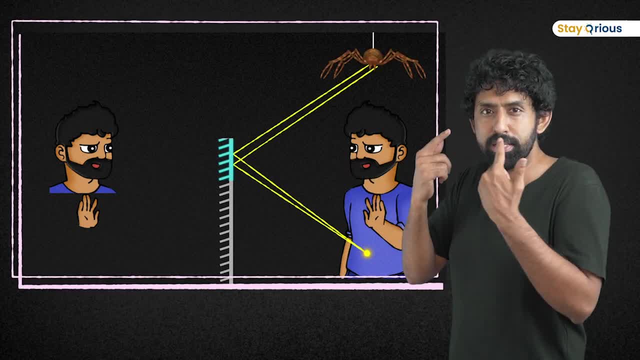 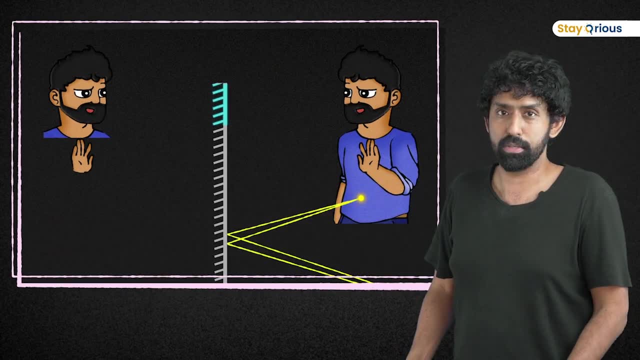 spider in the sky see my stomach but not me. Are they helping me see my stomach? No, Some of the rays or the photons go down and go that way. That helps some ant see my stomach but not my eyes. Only those that are hitting there and coming to my eye help. 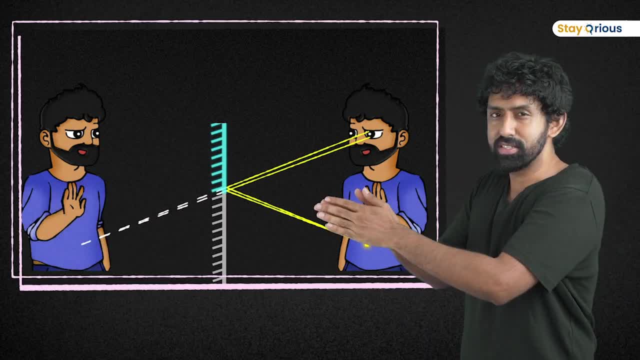 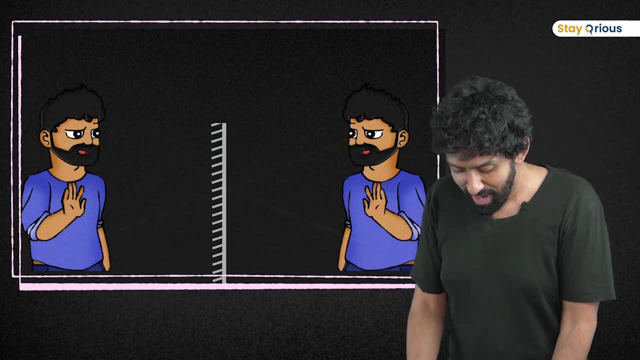 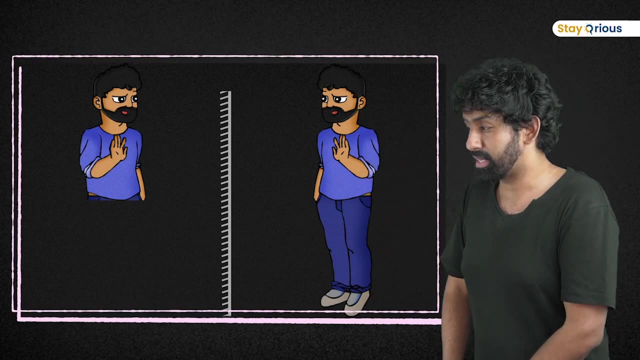 me see my stomach right, The ones hitting such that the angle of incidence equals angle of reflection- and coming and hitting my eye. yeah, Now you are ready to answer the question. how do I see my foot or my feet in the mirror? Light from some source hits my feet and then 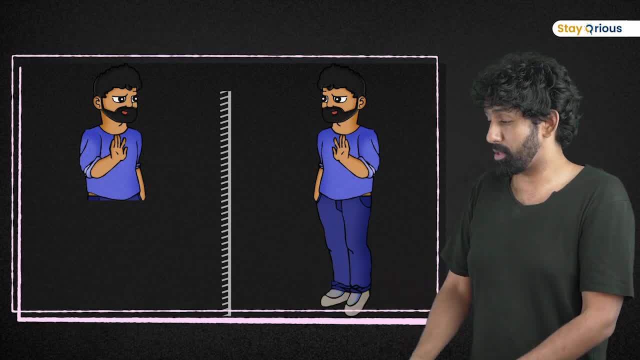 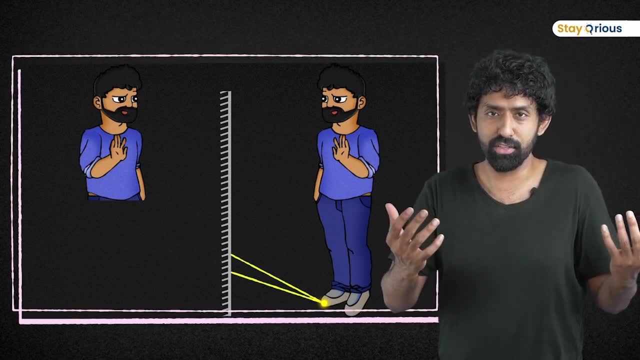 bounces off my feet and hits. Some of them hit the mirror, Some of them hit the mirror below there. Do those help me see my feet? No, because angle of incidence equals angle of reflection. You take that they bounce off that way they never reach your eye, It's. 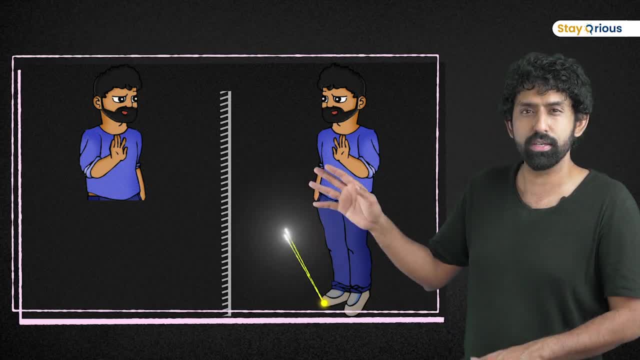 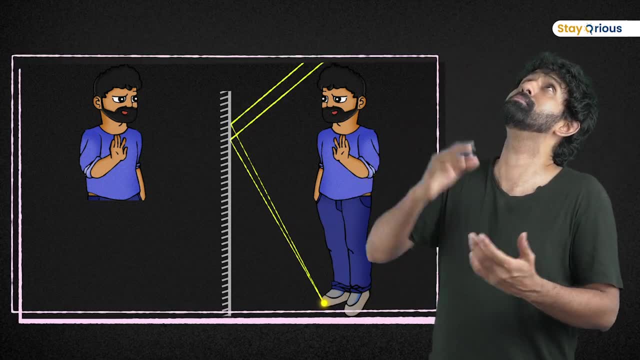 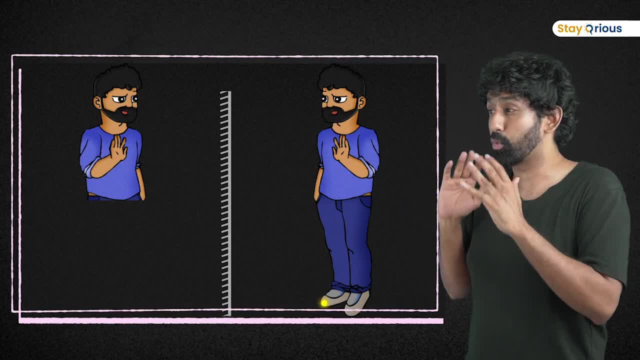 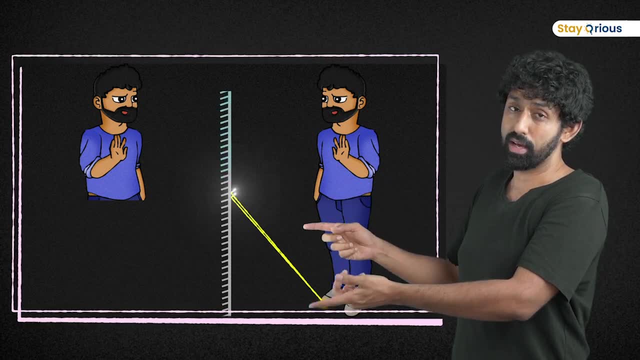 looking for those rays, not my eyes. The only rays that help my eyes are the ones hitting the mirror right in the middle over there, Because from my feet hit there, angle of incidence equals angle of reflection. hits my eye, creates an image of my feet right. 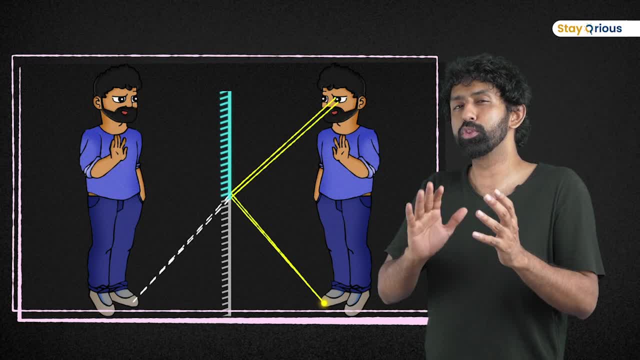 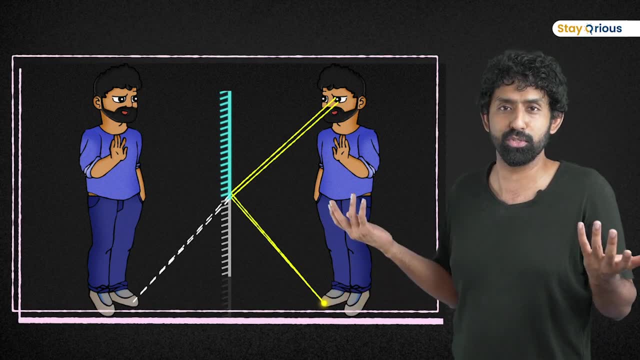 there, right behind the mirror over there, Only those rays help. Now, with that, you are ready to answer the question. What happens if I chop off the bottom part? Nothing, because it was not helping me anyway. Chop off a little bit more, nothing. chop off a little bit more. 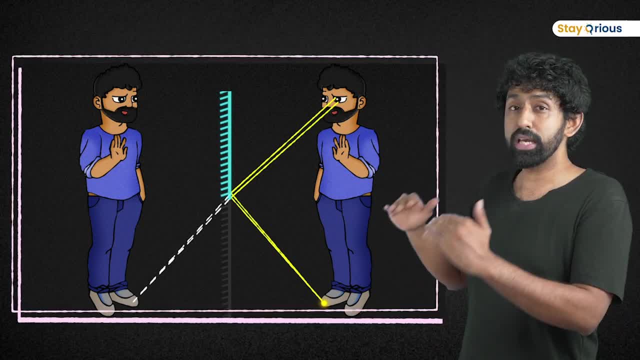 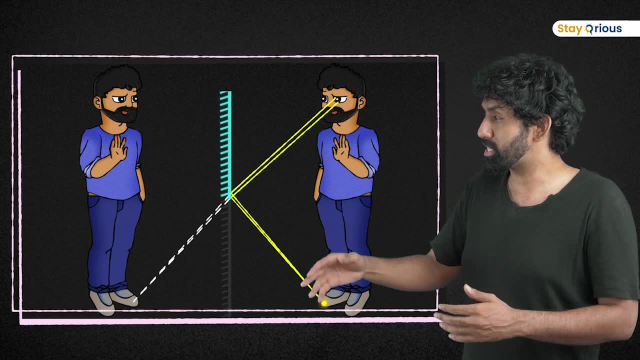 nothing until I reach the middle. Once I reach the middle, those are the rays that are actually bouncing off and hitting my eye. If I cut there, then what happens? Those rays have no mirror to bounce off of, So this is going to get absorbed in the wall and you can't see your feet, But you 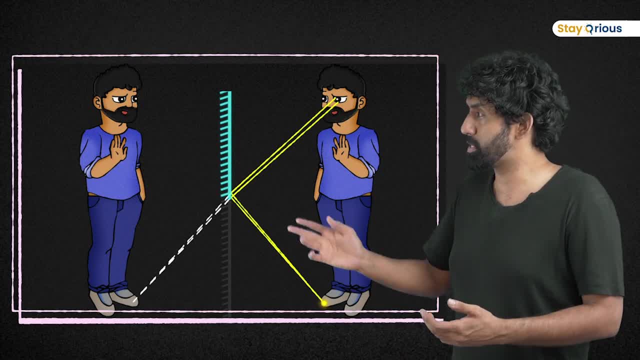 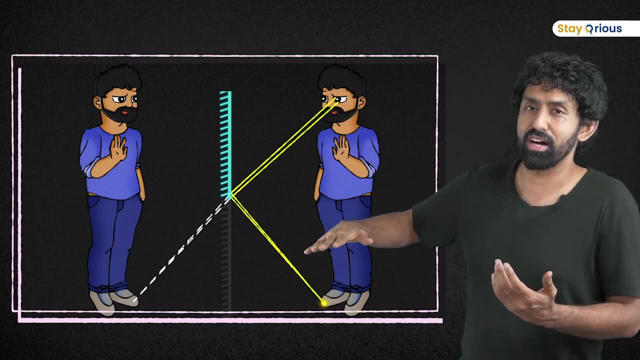 may ask: hey, what about those rays that will hit the mirror above that? Yeah, there will be some rays that hit the mirror above that, but will they reach your eye? They'll be going up. They won't reach your eye. So, exactly till half, you don't lose anything. The image formation will be. 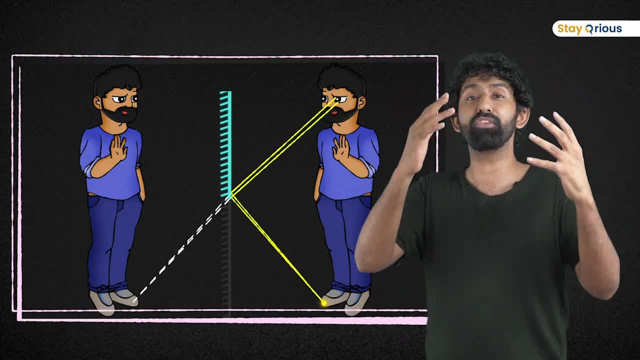 like this, But anything more than that. if you cut, you're gone, So you can safely cut half the mirror, and this is how you're seeing your image with a mirror.